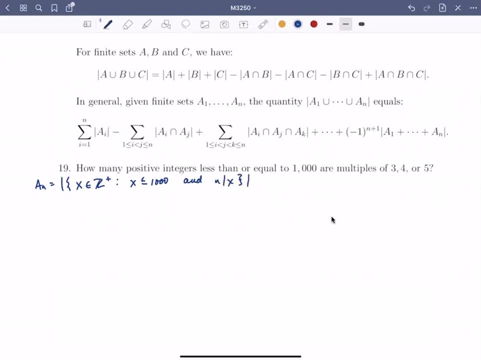 Okay, so that's what I'm going to use for our notation. A sub n, And we want to count. our job is to count A3, union, A4, union, A5,. right, We want to find the number of integers that are multiples of 3,, 4, or 5.. 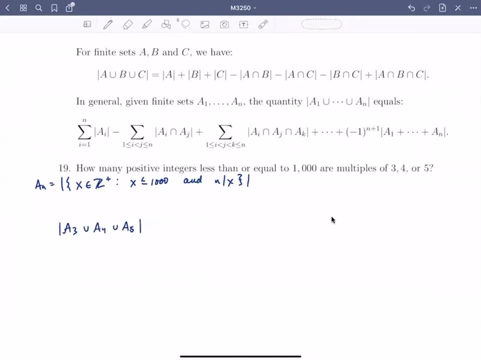 And this is classic inclusion-exclusion. So what we can do is we can add the individual cardinalities A3 plus A4 plus A5.. We're going to subtract pairs, So we're going to subtract A3 intersect A4, A3 intersect A5, and we're going to subtract A3 intersect- I'm sorry- A4 intersect A5.. 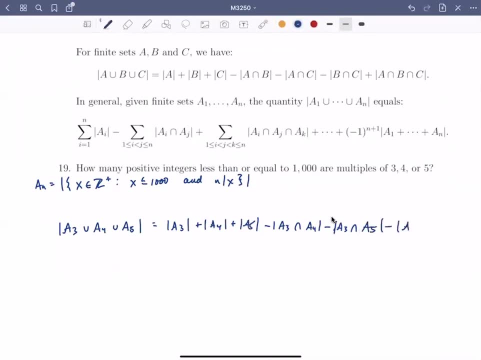 So let me write that a little better: A4 intersect A5.. And then we're going to add to that- I'm just out of room, but we're going to add to that the intersection of all three: A3 intersect A4, intersect A5. 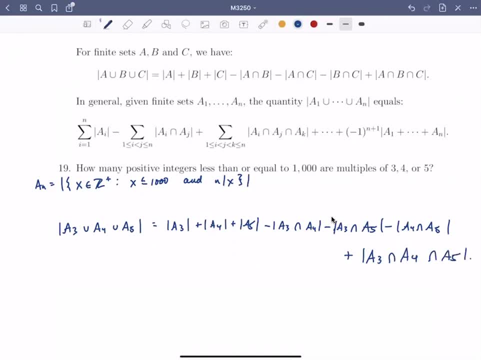 Okay, and so now what we need to do is we need to think about what are these sets? And, of course, when we take intersections, we're talking about ands. So for the first set, this is just- I'm just going to call it- A3,, A4, and A5. 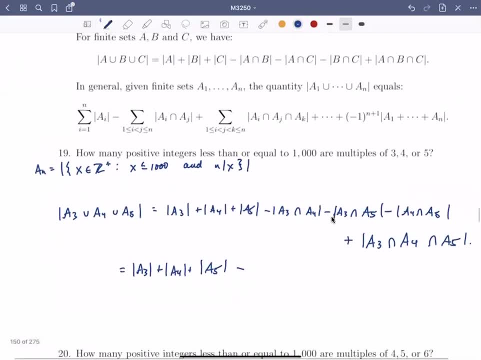 So A3,, A4, and A5. The second set. to be a multiple of 3 and 4 means that you're a multiple of 12, because that's the least common multiple, So let's say 12.. To be a multiple of 3 and 5 means that you're a multiple of 15.. 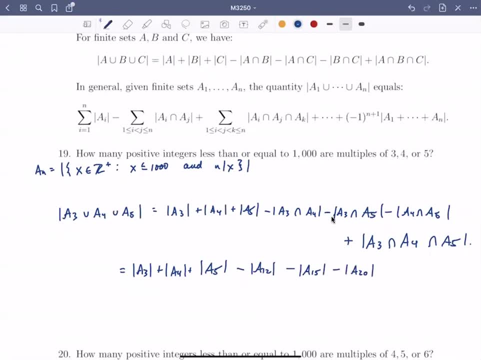 To be a multiple of 4 and 5 means that you're a multiple of 20.. And to be a multiple of 3,, 4, and 5 means that you're a multiple of 60.. Okay, and so we can add all these up. 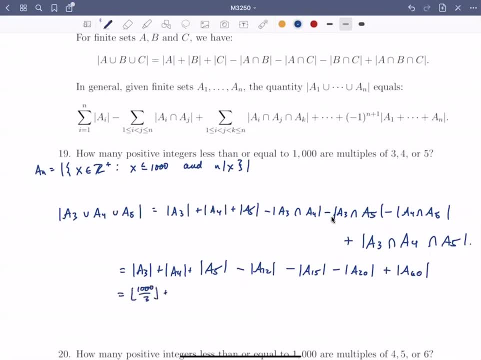 This is going to be the floor of 1,000 over 3 plus the floor of 1,000 over 4.. Plus the floor of 1,000 over 5,, minus the floor of 1,000 over 6,, 1,000 over 12,- excuse me- minus the floor of 1,000 over 15,, minus the floor of 1,000 over 20,. plus the floor of 1,000 over 60.. 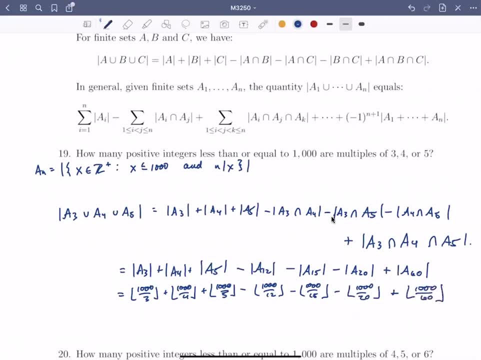 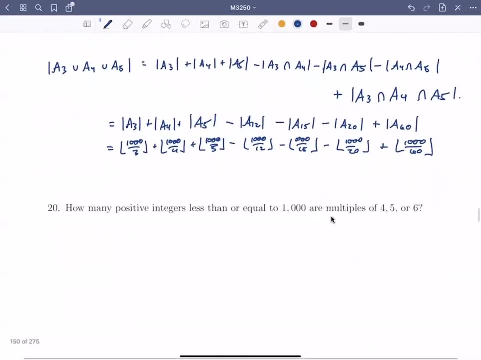 Okay, and so you could add all these up. I'll leave that to you: to add up and figure out exactly what you get. But that's how this would work. That's how inclusion-exclusion works. I'm going to do a similar exercise here. 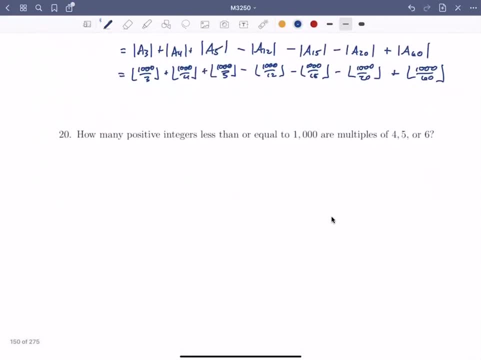 How many positive integers Less than Equal to 1,000 are multiples of 4,, 5, or 6.. Here, using the same notation as above, we're going to find the union, the cardinality of the union: A4, union, A5, union, A6.